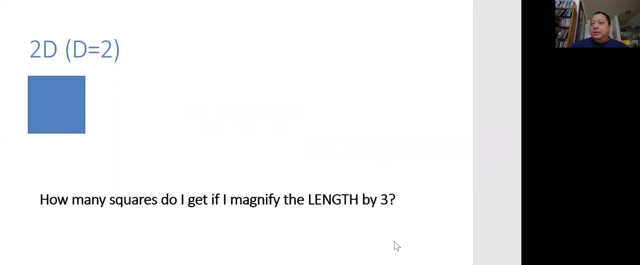 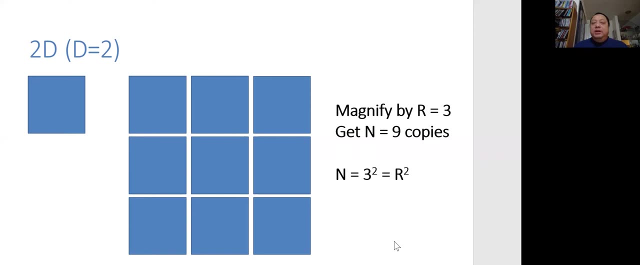 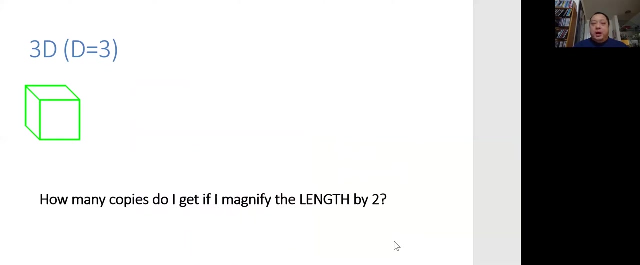 What if I magnify by three? Then I get three times three equals nine copies. I see that the relation is that n equals to r squared Three dimensions. now I have a cube block. How many copies? if I magnify the length by two, I get a larger block where each side is multiplied. 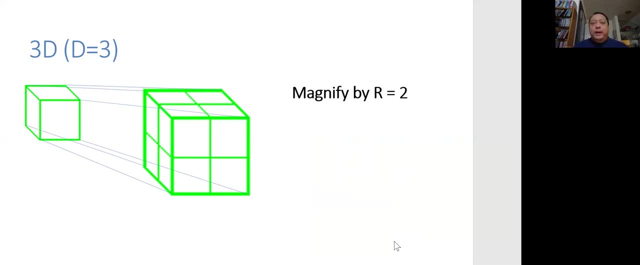 by two, It's a two by two by two. So I have eight copies in it And I see that relation is that n equals to r cubed. Let's try again with r equals three. How many copies do I get if I magnify the length by three? 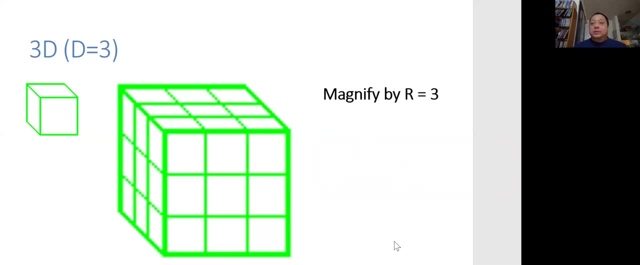 Then I have a huge block That's three by three, by three. Well, the top layer is three by three, so that's nine blocks, But I have three layers. So times three again equals twenty-three. So yes, I just verified that n equals r to the third power. 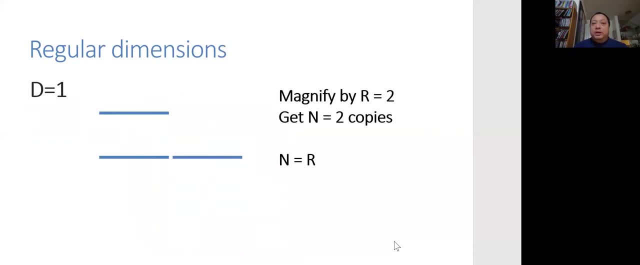 If I look back at the one-dimensional situation, I had n equals r. That can also be written as n equals r to the power one. So let's look at it. If I define the letter d as the dimension, then when d equals to one, 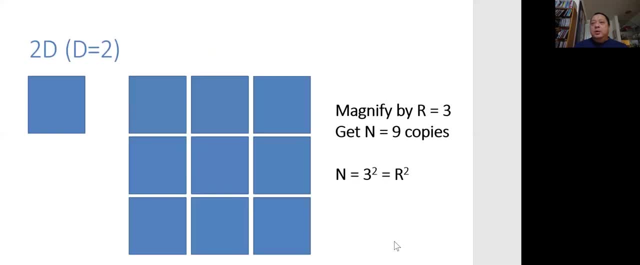 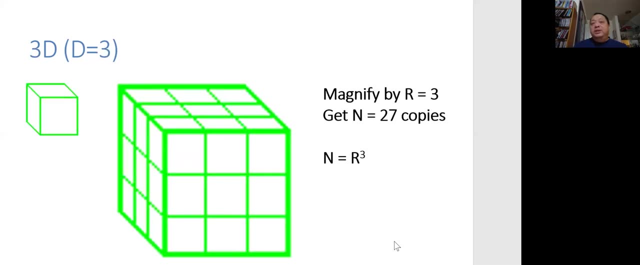 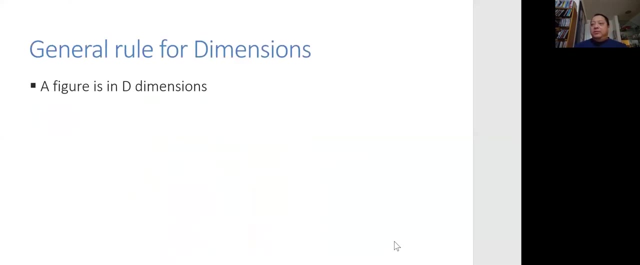 n is equal to r to the power one. When d is equal to two, n is equal to r to power two. And when d is equal to three, n is equal to r to the power three. So the general rule is that if I have a figure in d dimensions and I magnify by a factor of r, 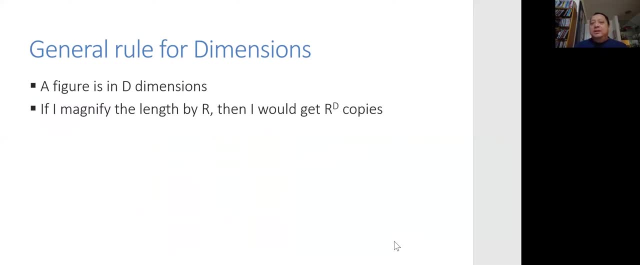 then I would get r power d copies. The relationship is: n equals r to the power d. So I'm ready for my secondBER. Let's do it to compute the formula for d. I can start with the relationship: n equals r to the power d. 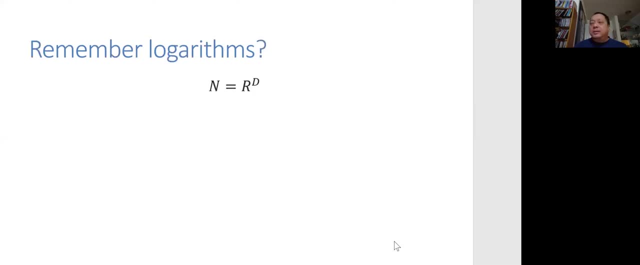 and I isolate the variable d. For that I need logarithms. So I go through some algebra and I end up with: d equals log of n divided by log of r. So that's the dimension formula. I define r and n according to what I've been doing. r is the magnifying factor. How much do? 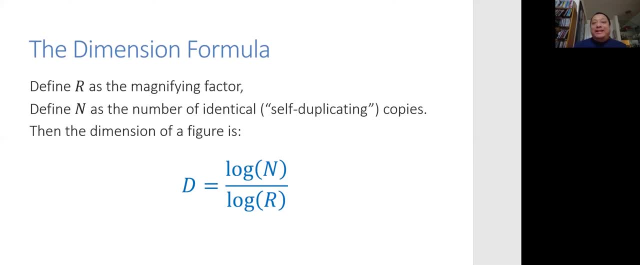 I magnify by, And n is how many identical copies I get. Then d is equal to log of n divided by log of r. So I'm ready now to compute the dimension of a fractal figure. Let's take the Koch curve. 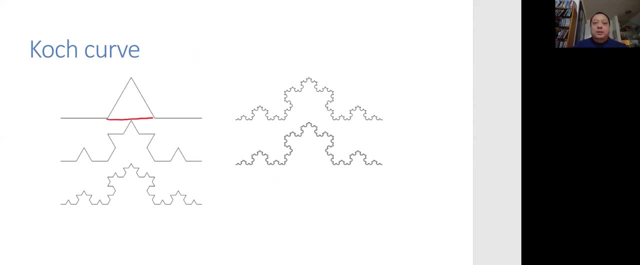 also called the snowflake curve. The Koch curve starts with a line. I punch a hole in the middle- one-third of it, and I put two sides of an equilateral triangle in its place. That gets me the first generation of the Koch curve. It has four line segments. so in each of those four line, 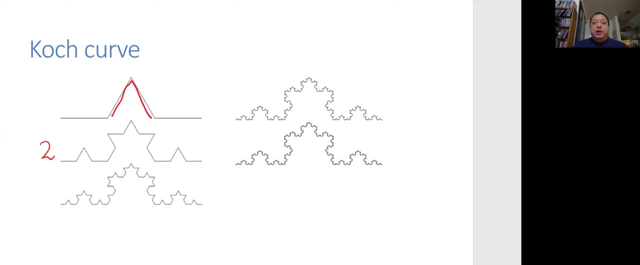 segments. I will do it again. I put a hole in the middle one-third of each line segment and I put two sides of a triangle in it, and I do it again and again, and again and again, all the way to infinity. So the question is, how many identical copies do I have? I put a hole in the middle one-third. 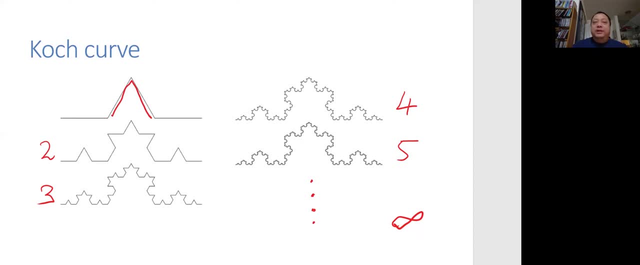 of the triangle. I put two sides of the triangle in it and I put two sides of an equilateral triangle, and I put two sides of an equilateral triangle in it and I put two sides of an equilateral triangle in it. So the question is: what is the dimension of the Koch curve at infinity? So let's do the. 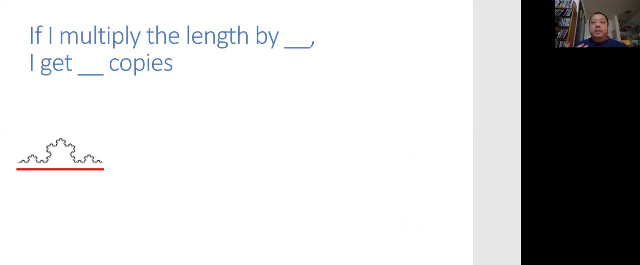 same thing as before. If I multiply the length by blank, I get blank copies. What should the first blank be? Well, since the snowflake curve is built by cutting out the middle one-third, it's logical that I should use the number 3 for r. So I have a length that is three times the old length. 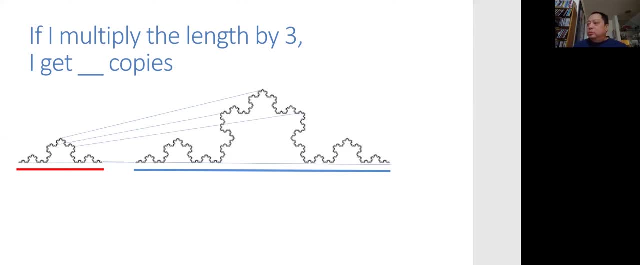 and I magnify the Koch curve curve How many copies of the original one are in the big magnified version? Four copies. So my r is 3,, my n is 4, and I plug it into the d-formula: g equals log 4 divided by log. 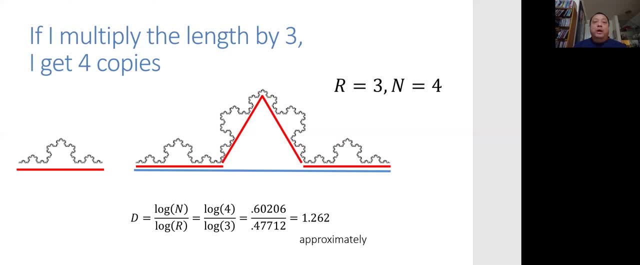 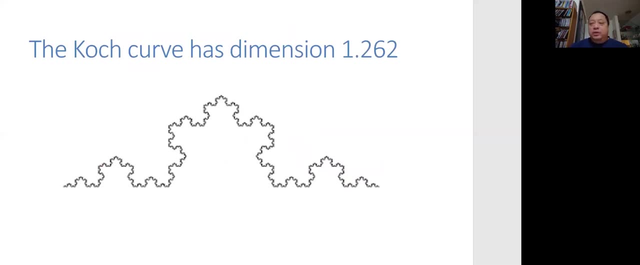 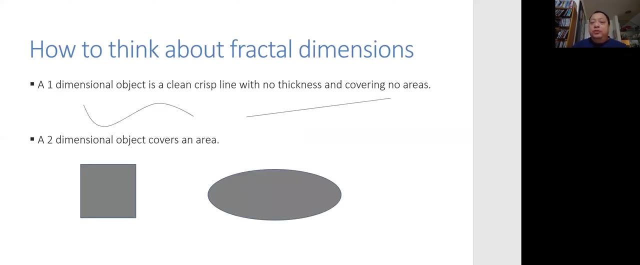 3. I get my calculator and I get 1.262 approximately. So that means the Koch curve has dimension 1.262.. It's a dimension with decimals. So when I first learned of fractal dimensions I was excited, Excited that I'm no longer bound by the whole numbers. But I had a hard. 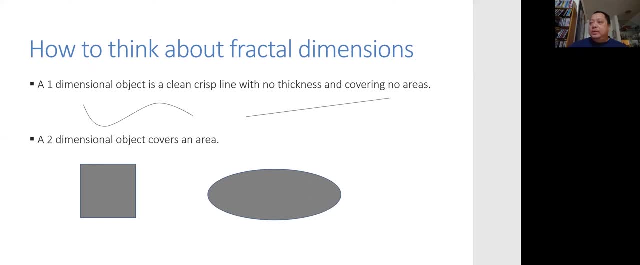 time imagining why it is that way. So here's how to think about fractal dimensions. A one-dimensional object is something that moves along in just one path. You may, But you're still moving along just one path. It's nice, clean, crisp line, with no thickness and covering no area. 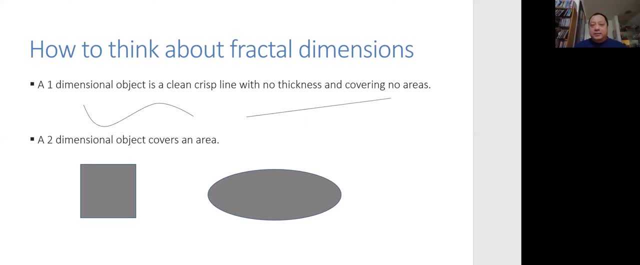 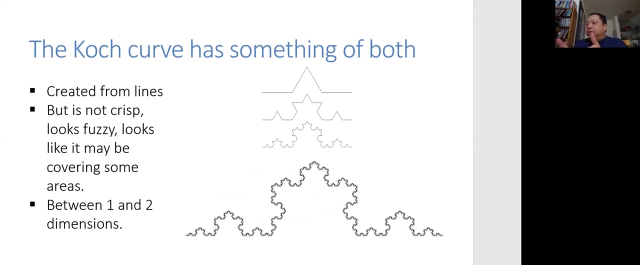 A two dimensional object covers an area. It could be a circle, it could be a square, any figure, But it covers an area and that's what makes it two dimensional. Well, the Koch curve has a little bit of both. When we create the Koch curve, we create it by just drawing lines. 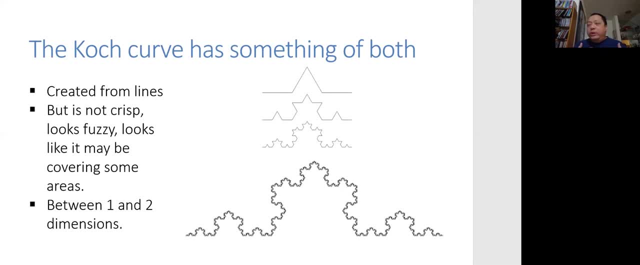 We're not coloring in any area. But when we keep doing this and we get to infinity, then the final product doesn't look crisp and clean and doesn't look like someone just traveling along a path. It looks fuzzy, It looks like it may be covering some area. 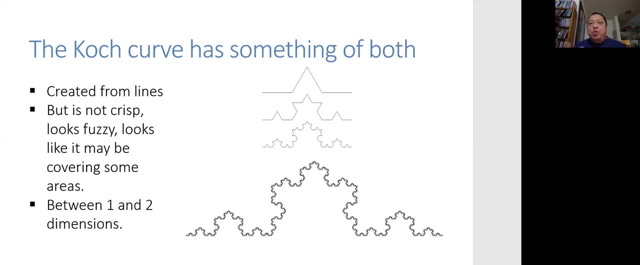 But it's not. So it feels like it's something more than one dimension, But it's not quite two dimensions, because we know it's not an area, It's just a bunch of lines, An infinite number of line segments. So that's the key, because an infinite number of tiny lines make the fuzziness and it makes the figure into something more than just one dimension. 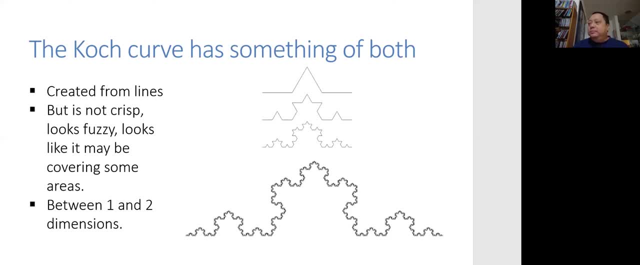 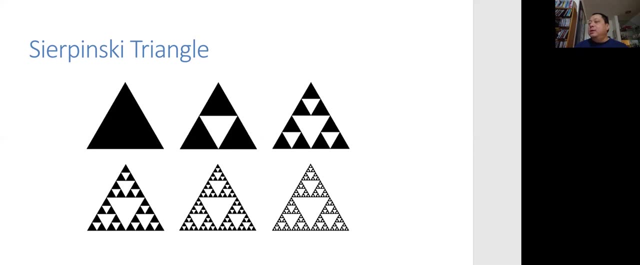 Less than two dimensions. So it's one point something. So let's do another example. This is the Szypinski triangle. We started with a triangle, or collodion is in two dimensions. Then we punch a hole in the middle of it. 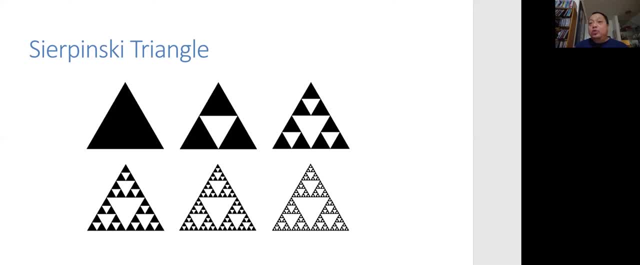 That gets us three little triangles, which we then punch a hole in the middle of them again, And then we repeat, and we repeat to infinity. If we keep going to infinity, then think about it like this: If there's any solid part left, we would be punching a hole in it. 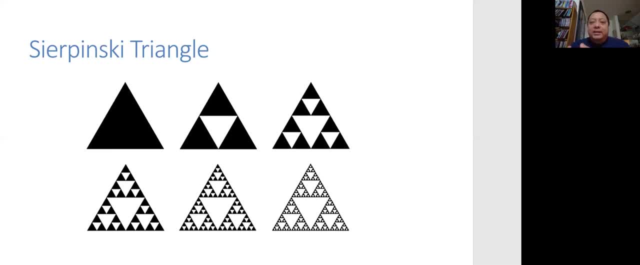 That means it feels like by the end there will be just an infinite number of lines with no areas. So it seems like it's lost its second dimension. But to call it one dimensional is also unfair, Because in another way, no matter how much you punch a hole in the triangle, there will still be some triangles left.